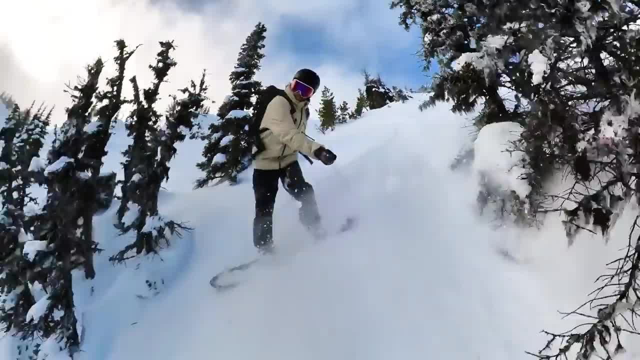 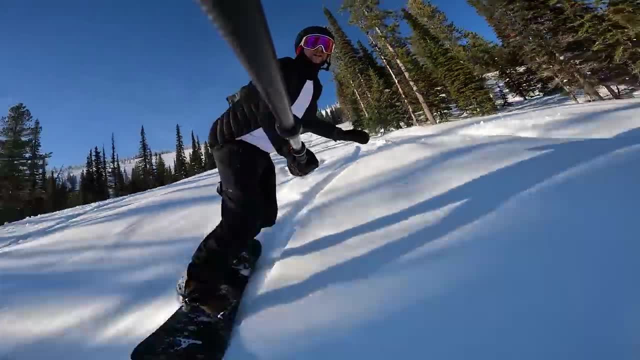 that I'm riding with speed. I'm looking ahead, I'm seeing where I need to make turns, where I need to slow myself down, where I can pick up speed and any hazards that may be along the way. By looking ahead and planning out your turns, you're going to be able to ride with. 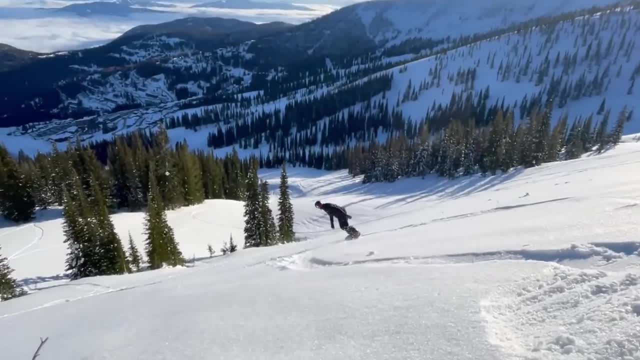 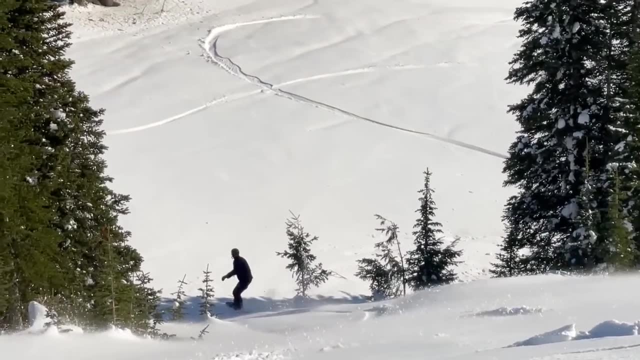 more speed because you'll know all the obstacles that are coming. It's going to keep you safer and it's going to give you that confidence to pick up speed where you need to. You can really get into trouble if you're riding with speed and there's an obstacle or something unexpected comes out in. 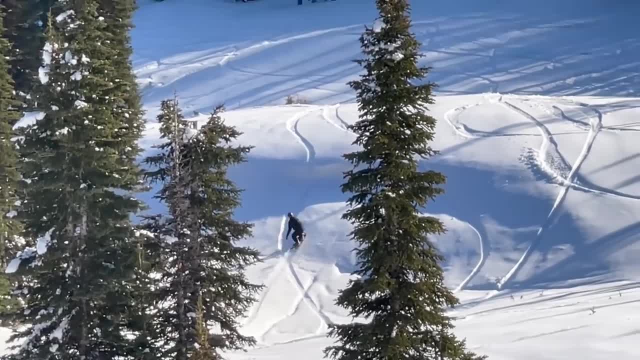 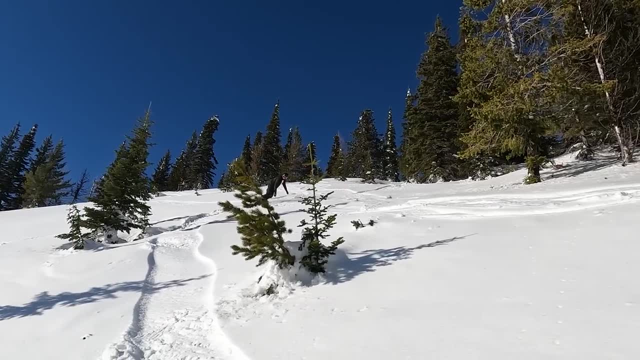 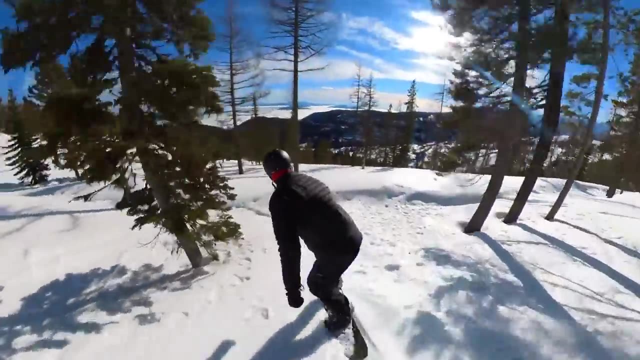 the way of your riding. So by always planning it out, looking ahead, it'll help you to avoid those obstacles and ride much safer. The next thing you need to add into your riding is the ability to do different turn shapes depending on the terrain. In this video I'm snowboarding at Mount Schweitzer and the conditions. 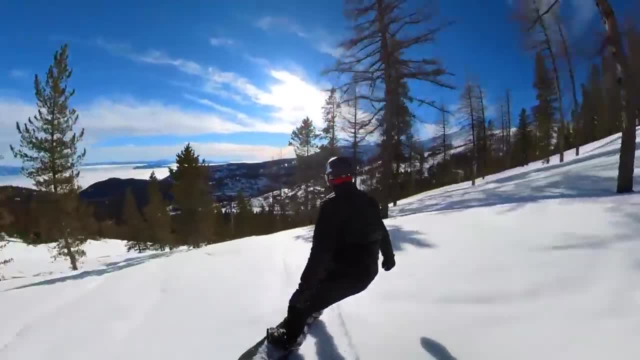 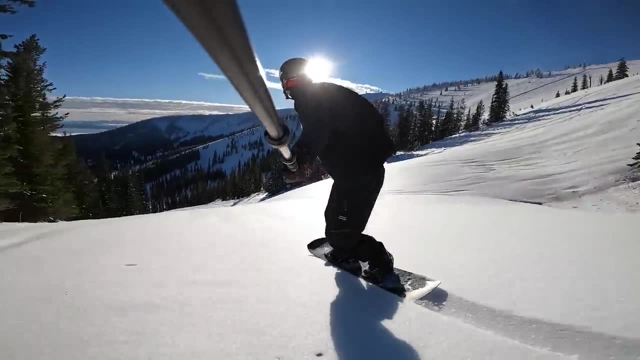 were really all over the place in terms of terrain and snow quality, and I was always adjusting my turn shape depending on those factors. In the areas where it was really wide, open and mellow, my turns were big, allowing me to pick up more speed with those big and wide turns In areas where it was. 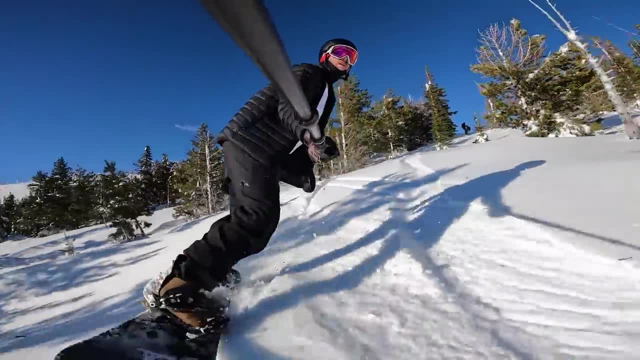 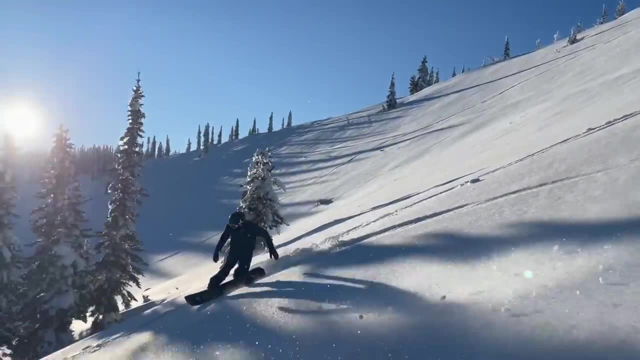 a bit more tight. I was doing quicker, fast turns allowing me to quickly maneuver through trees while maintaining my speed, and in other areas using a combination of both, So quick turns where I needed to, and then wide open ones to pick up speed or maintain my momentum. So it's really 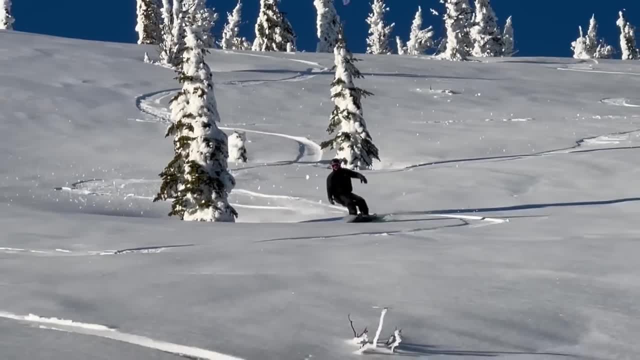 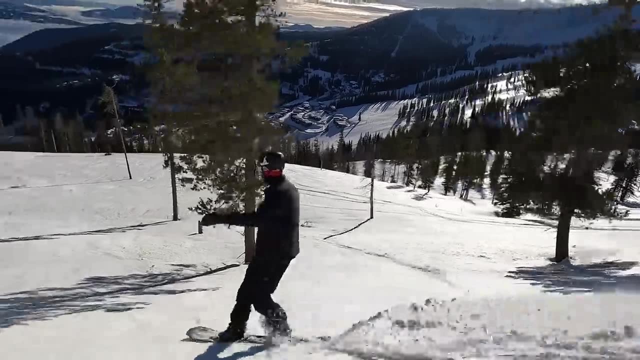 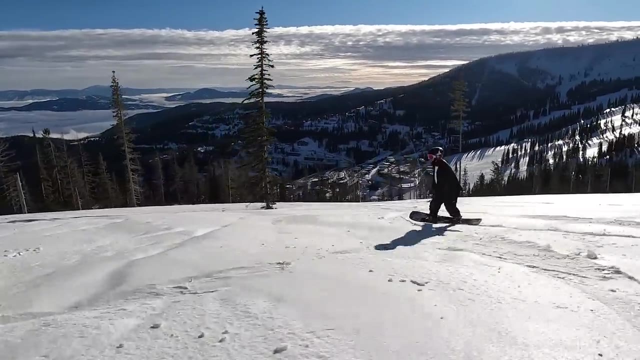 important, if you're riding with speed, to have a wide variety of turn shapes to allow you to adjust to the terrain and conditions. Another important factor for riding with speed is being able to control your speed. to control your speed equally on both your heel and toe turns. As you go through each turn, you're 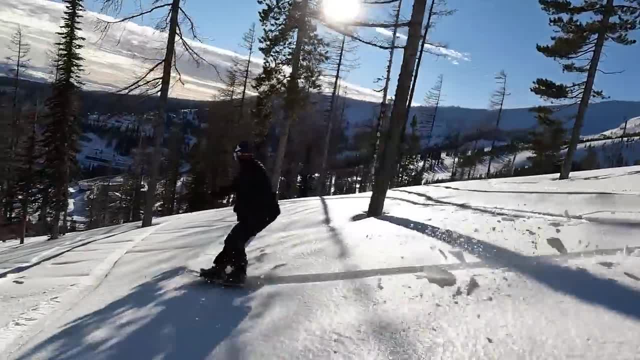 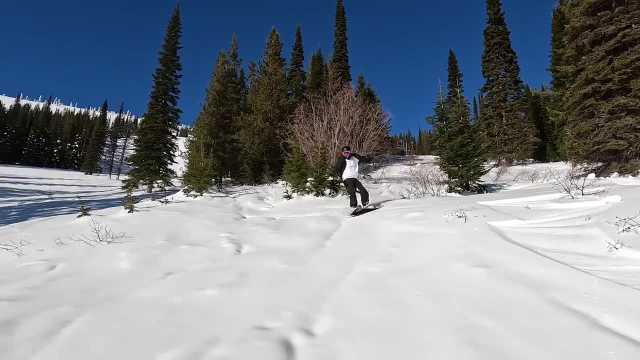 spraying a little bit of snow or putting some pressure on your snowboard to control your speed a little bit. If you feel like one edge is weaker than the other, then what happens is you always have to compensate for that weaker edge by controlling your speed more with the stronger one, By not 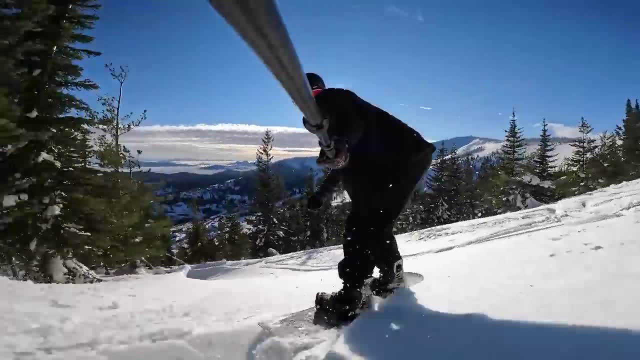 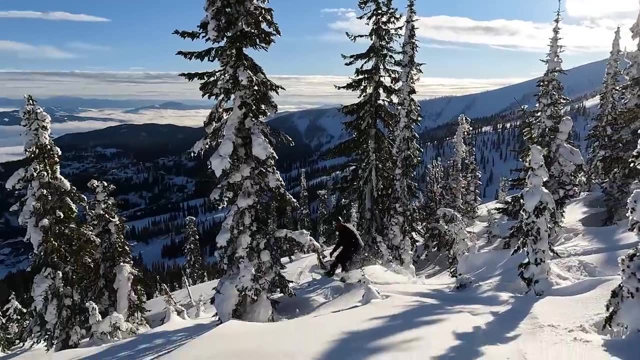 being able to confidently control your speed equally on your heels as toes, then you're not going to be able to ride with a good flow and it's going to limit the amount of speed you can ride with. If this is a problem you can feel in your turns, take your riding someplace that is less.